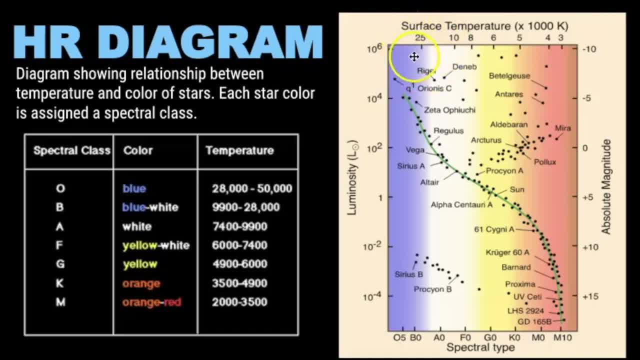 over here. This is up to 25,000 degrees Kelvin, or it can actually get higher than that as well Along this axis. this measures luminosity, So bring your attention right here. This is luminosity measured in suns, So if you come to the one and march yourself over here, you can find. 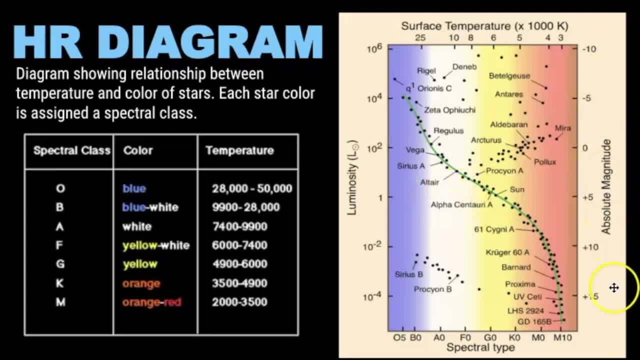 the sun. Absolute magnitude is just another descriptive way to measure brightness, And then at the bottom we have spectral type or spectral class, And the different letters represent different color and temperature ranges. And these are. these can actually be broken down into like 01, 02,, 03, 04- stars describing how hot. 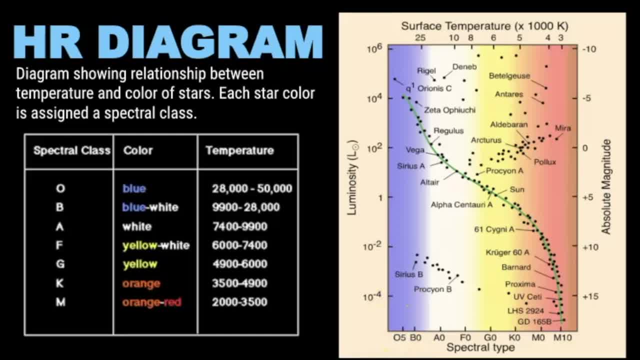 they are and their different colors. So here I listed what the spectral class is, what the color would be and then what the temperatures would be as well. There is a mnemonic device that is used to help you remember what the spectral class is, And that is OBA, fine. 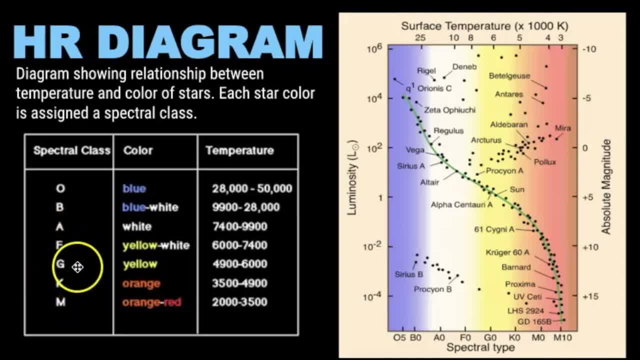 girl kiss me, or you can use guy instead of girl, whatever helps you remember, But that mnemonic device can just help you remember what the temperature is And then at the bottom you can see what the spectral class is. Before we move on, I would like to tell you more about the 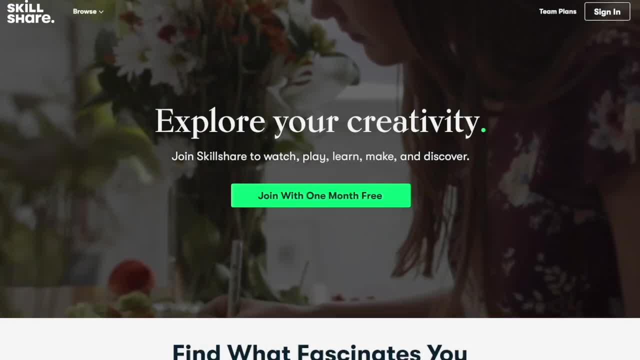 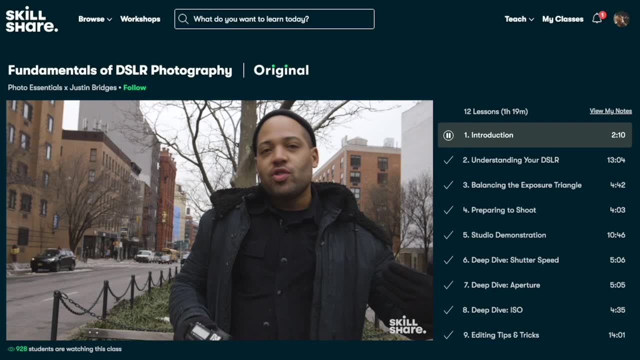 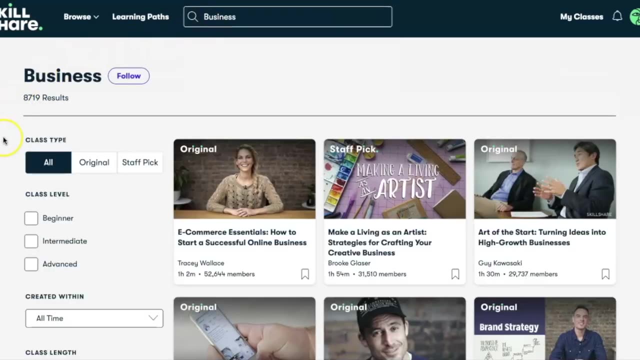 sponsor for this video: Skillshare. Skillshare is an online learning community with a wide variety of tutorials. These are video based quality lessons that can teach you anything from photography to business skills, to cooking or even animation, And they're really good, practical. 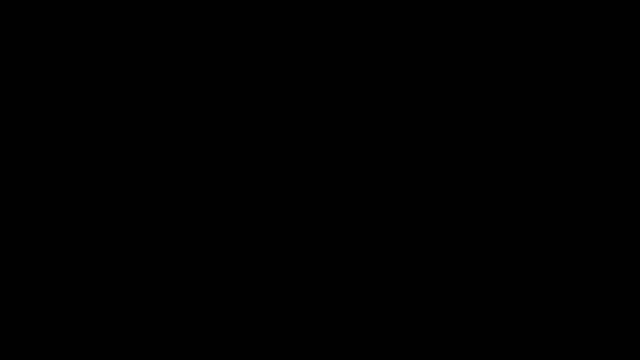 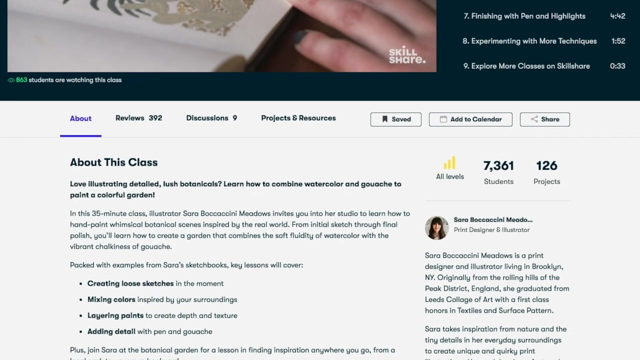 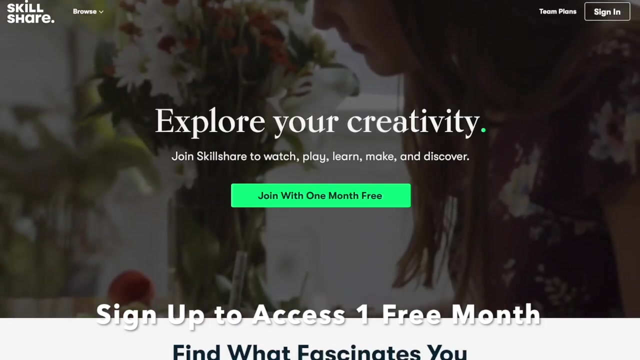 courses, And even though I'm a professional educator, I'm also a major believer that you can acquire any type of skill on your own outside of a formal environment. So there's a link in my description and the first 1000 people to use the link will get one month free trial of 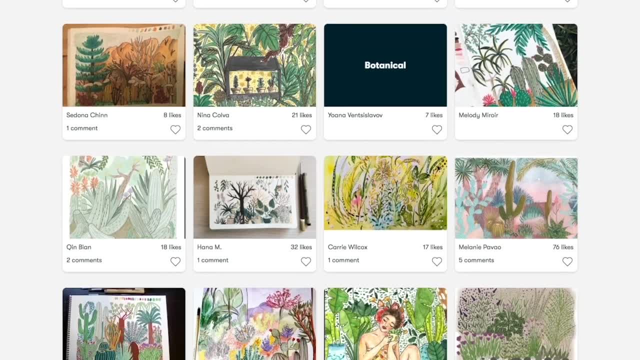 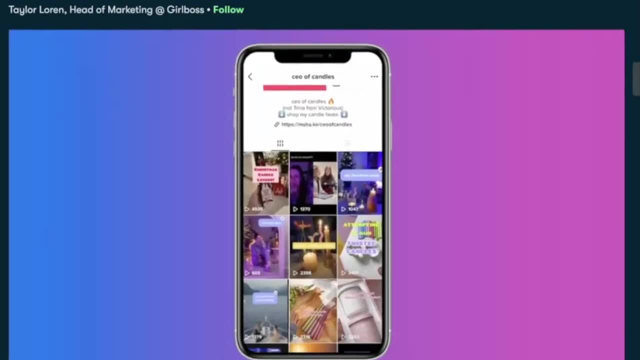 Skillshare And it's a really great deal, So go click the link and take a course For me. I've been using Skillshare to learn how to reach a greater audience through new platforms like TikTok. This has been a huge transition for me, and the course called Mastering TikTok- 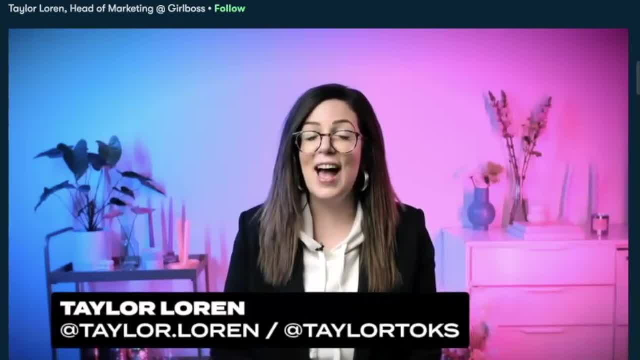 by Taylor Lauren has really helped me to face my fears and just get my content posted. I've been making videos a particular way for many years And this course was able to guide me through this new platform, So I highly encourage each of you to use my link and check it out. 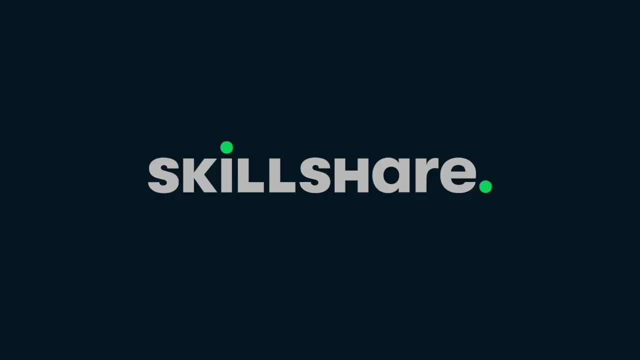 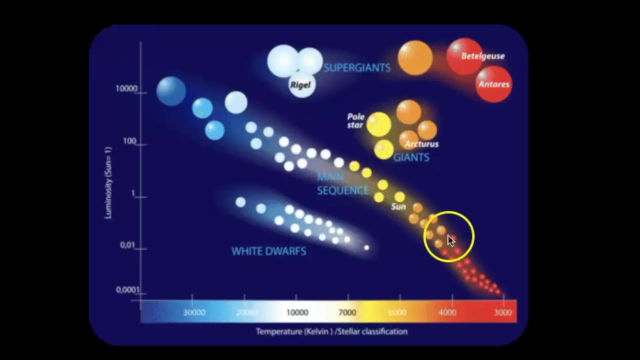 And remember, self growth is achievable through Skillshare. Another important concept to understand about the HR diagram is what each of these categories mean in terms of stellar evolution. So first here, this long band that goes from the upper left all the way to the lower right. This is called the main sequence. 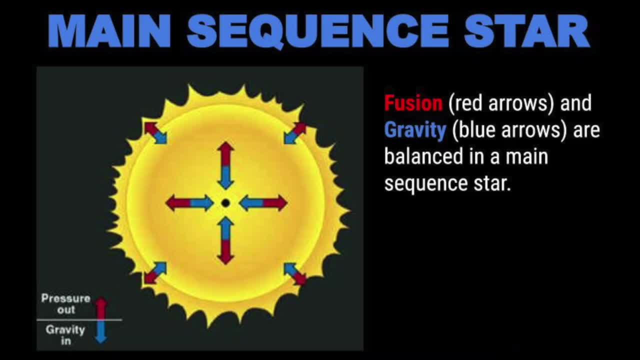 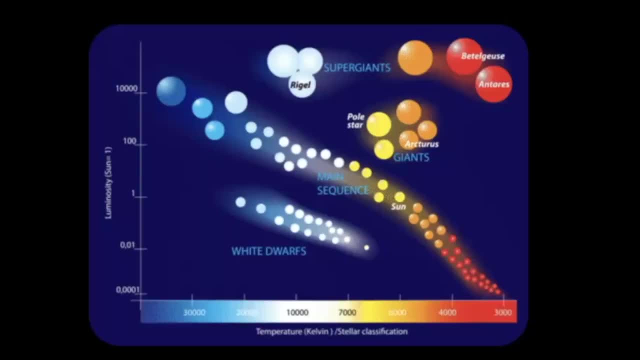 band, And this is where stars spend majority of their life. they are stable in terms of the pressure from fusion and gravity, pulling everything to the center, So it's a balanced star. But over time, a star's position on the center of the star is going to change And that's going to 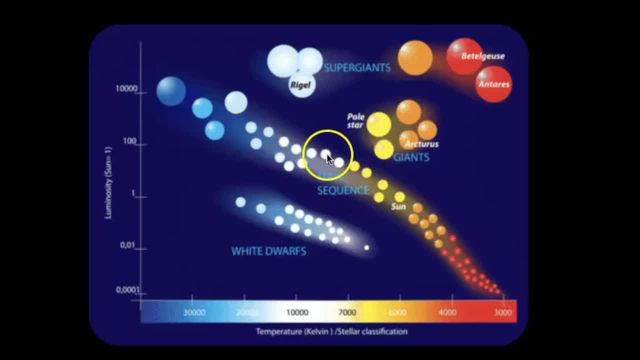 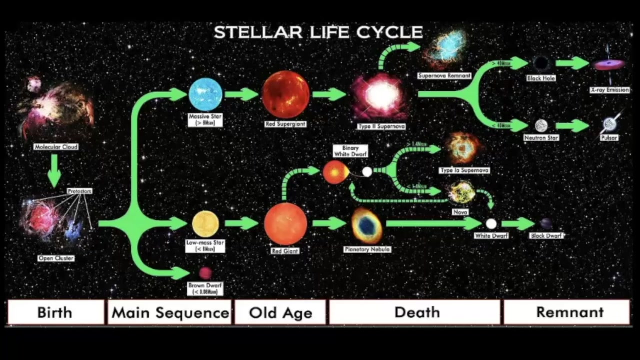 this diagram will change. They begin as main sequence stars, they evolve into giants or maybe super giants, And then eventually they fizzle away into white dwarfs. And to understand this, you need to understand the life cycle of a star. Now, eventually, I will be doing a longer video. 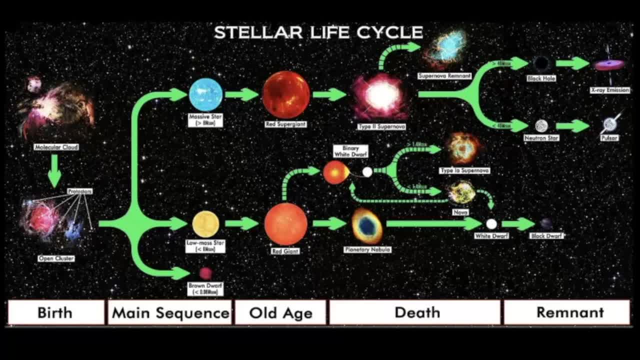 on this process, But I can briefly go over it so you can understand how a star's position on the HR diagram will change. So all stars are going to change And then eventually they're going to begin in molecular clouds with hydrogen and dust And eventually something hits this molecular cloud. 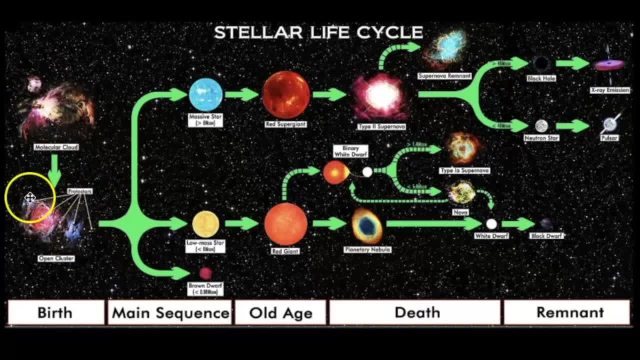 perhaps a shockwave from a distant supernova, And then proto stars begin to form, And most stars, all they form within clusters that are hidden inside these, hidden inside a nebula. So once a certain temperature hits, these or the stars reach a particular temperature, they begin to form, And so 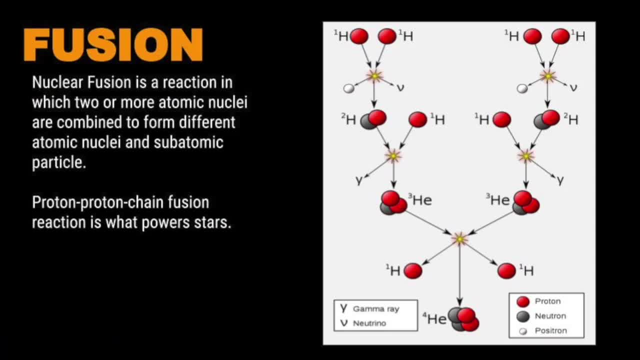 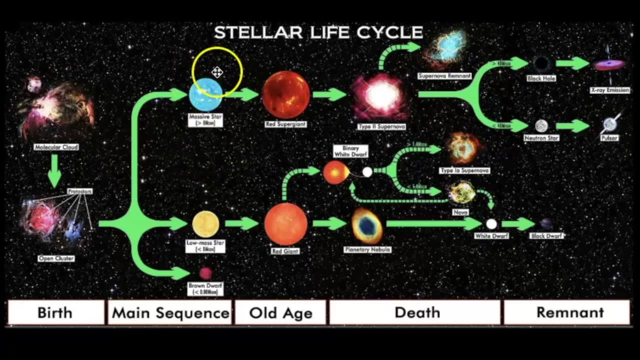 the process of fusion begins, And then this is when stars become a main sequence star. the process of fusion is happening. stars are fusing hydrogen into helium and we can have really massive stars that are typically blue in color. Or you can have a low mass star like our sun, or even a red dwarf star. 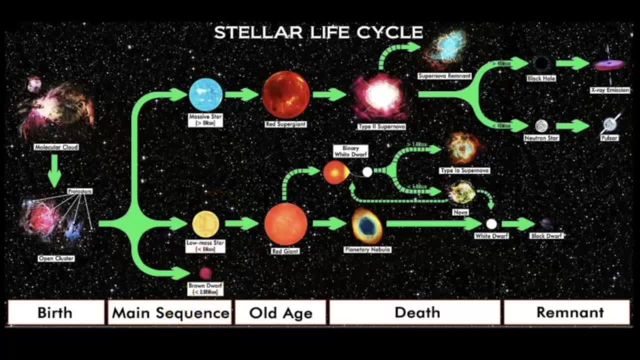 Brown dwarf stars are essentially failed stars that never got hot enough to start the process of fusion. Over time, though, as a star starts to fuse up all its hydrogen and it starts to fuse heavier elements, the star enters its old age cycle. If it's a massive star, it'll turn into a super giant. 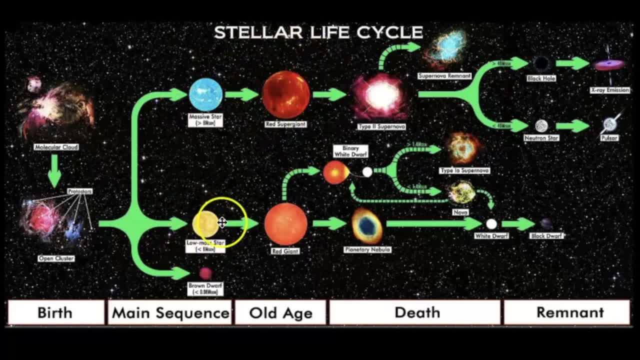 star. If it's a low mass star like our sun, it'll turn into a red giant, So it grows in size And then over time you have eventually all the gases. there won't be enough mass. there won't be enough. 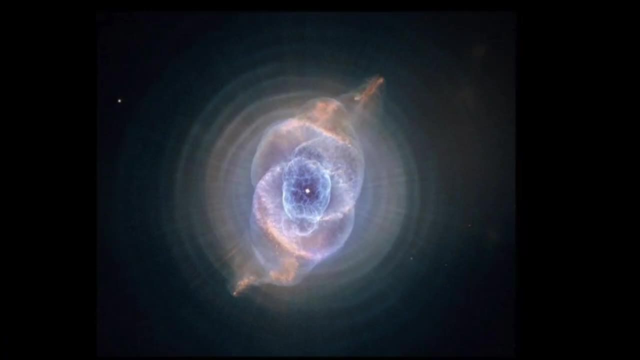 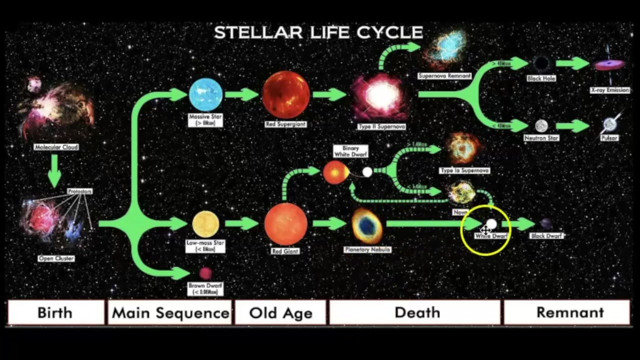 mass to continue fusion, So it starts to fizzle away into these beautiful objects called planetary nebulas And then it turns into a white dwarf. And a white dwarf is essentially a hot leftover core of a star. It's really really hot, It burns. it's not too bright because it's just small. It's very. 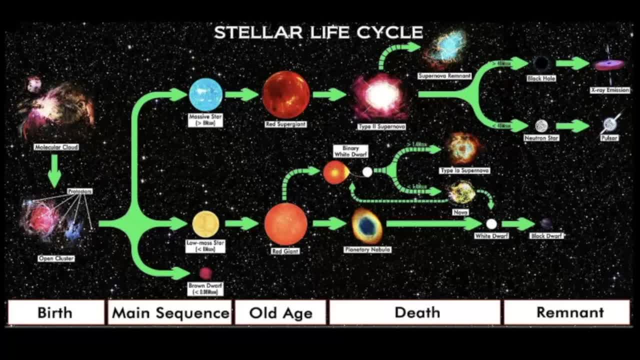 small So, but very hot, and eventually it fades into a black dwarf. But if you're a massive star, like a star like Betelgeuse or Rigel and Orion, what will happen is this star will become unstable iron. 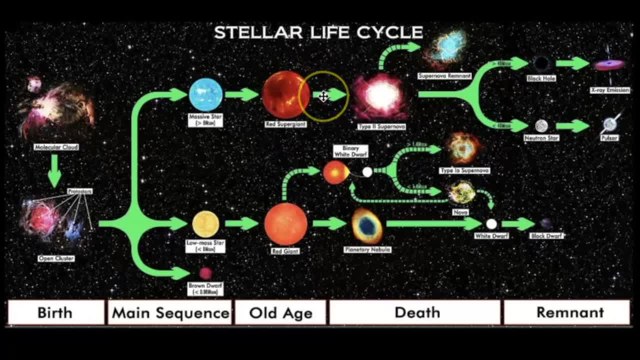 forms inside of it and it turns into a supernova And then, depending upon its mass, it'll either either turn into a black hole or a neutron star. So some of these objects that I'm circling right here they aren't really seen on the HR diagram, But this pathway we can see some of these stars. 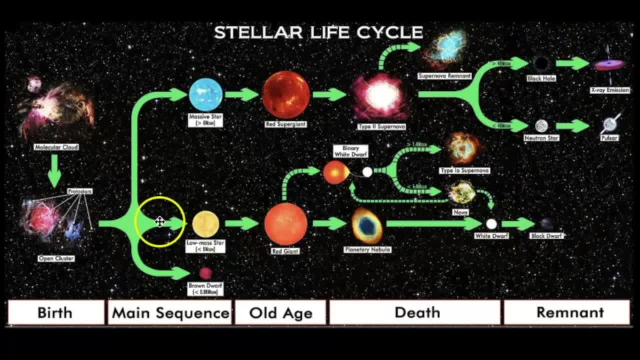 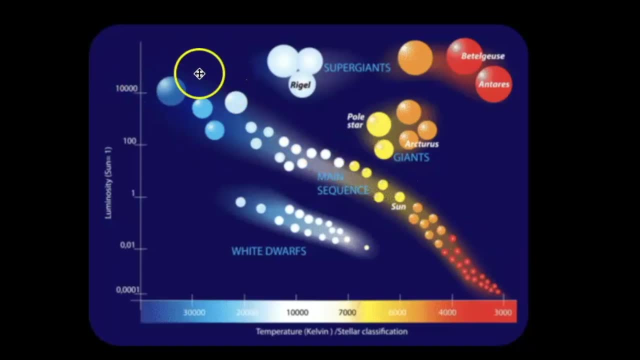 So, bouncing back to the HR diagram, I know that was like a really quick description of stellar evolution. There's a there's a lot more to say in on that topic, But that that will be for a later video. So here are these main sequence stars. Here we have these as giant, like blue, giant stars. 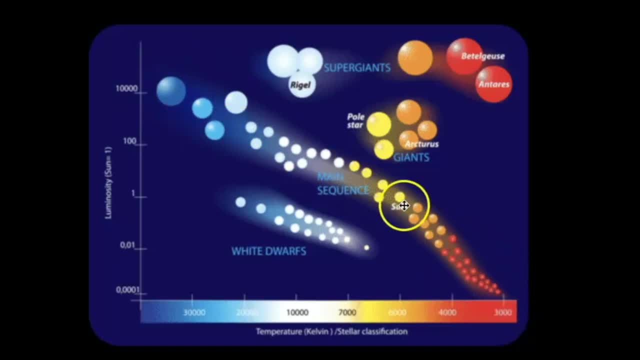 And then down here we call these red dwarf stars, And these are. these are stars like our sun, And then what happens is as they start to change, they start to change And then, as they turn into a to run out of fuel, stars in this area will evolve into giant stars, so they're starting to grow in. 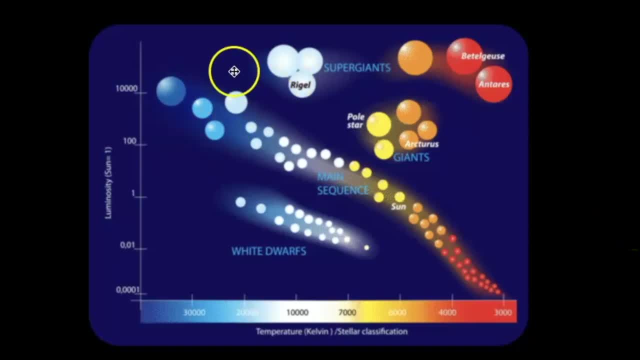 size. but stars in this arena, on this part of the main sequence band, will grow into super giants. they'll get really, really big and some of them will cool down, others will still stay relatively hot, but then, as these red giants fade over time into planetary, uh nebulae you, they will eventually. 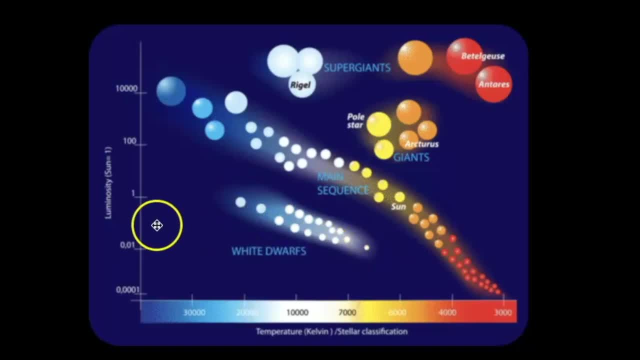 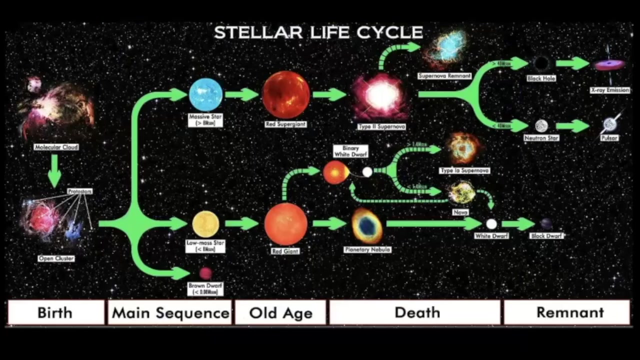 turn to white dwarfs and you can see they're. they're not as bright as the sun because they're lower in terms of luminosity, but they're still really, really hot. so i hope this helps you kind of understand the process of stellar evolution and how a star's position. 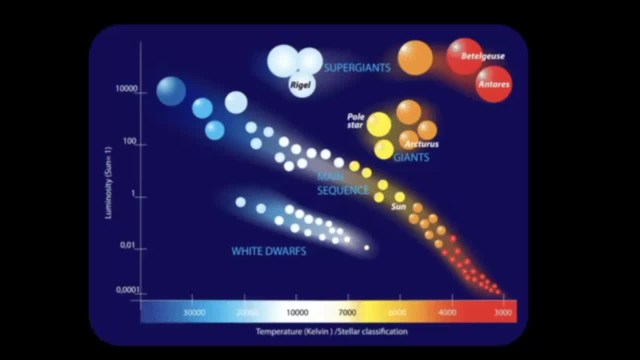 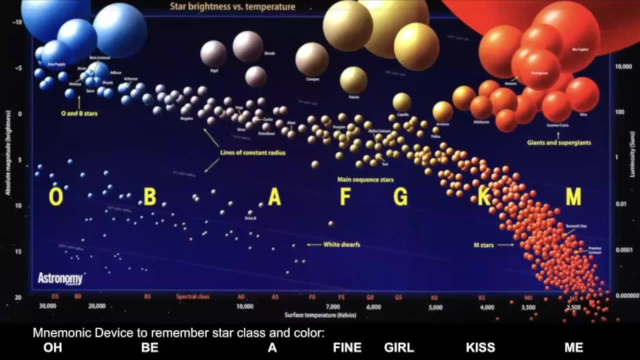 on this diagram will change over time. this is another version. i'm trying to show you as many versions as possible about the hr diagram. like this one because it incorporates size here too, which is something you have to consider, because if you look over here, this is the main sequence band And this is where stars spend a. 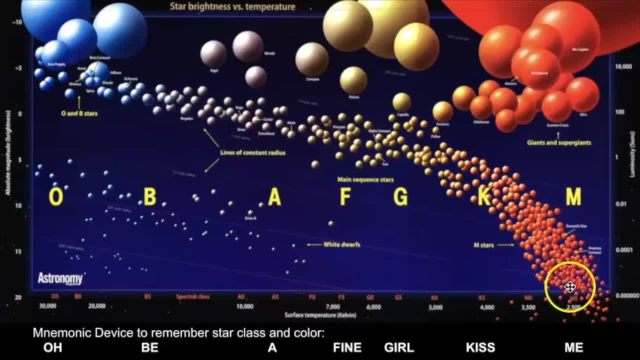 majority of their time on the HR diagram, And what this means is that they are balanced with the force of fusion, along with the force of gravity. So these are everything in this band. here is a stable star, But red stars just aren't small. they can also be very big, but they could still be the 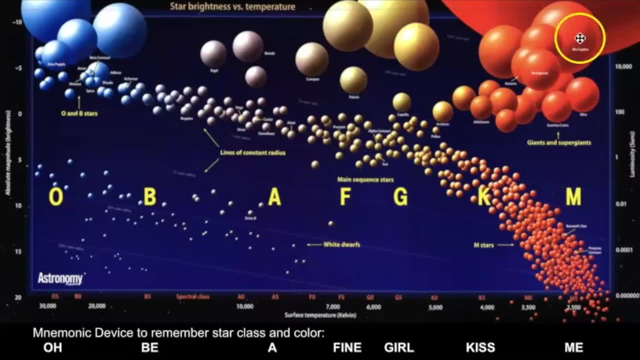 same color and temperature, which is really, really fascinating to me. Now, as a star gets older, depending upon the size that it is and upon its mass, it will change differently throughout its life. So here we have F and G, main sequence stars. these eventually turn into red giants. 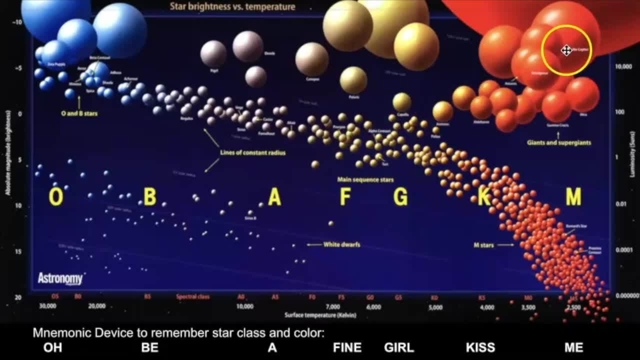 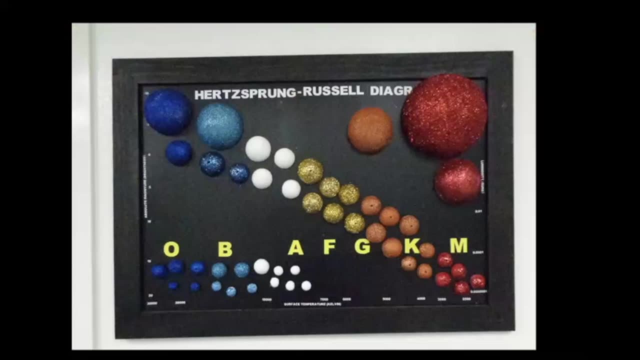 stars up here will turn into super giant stars, which means that the location of fusion starts to change and the types of elements that are being fused changes as well. What's really fun about the HR diagram- at least in my classroom- is I had the chance to make it into a physical 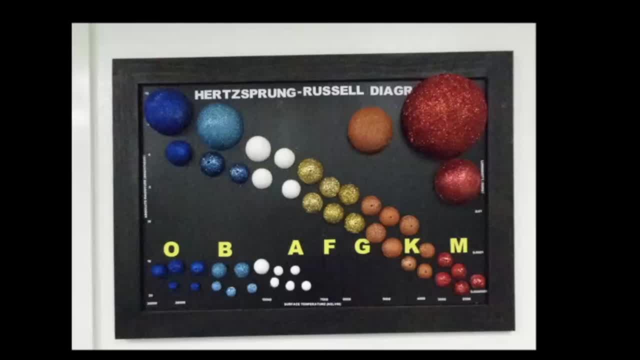 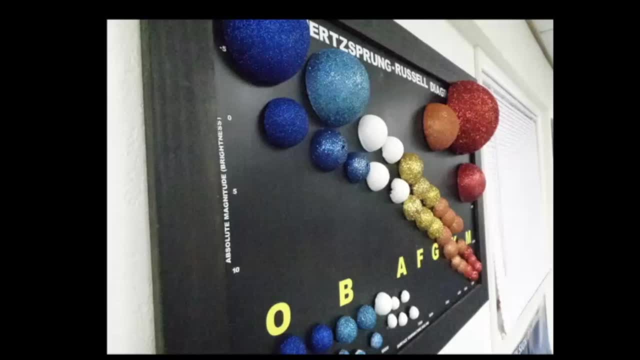 3d model. And we did this by having cutting apart styrofoam balls, and then we gave them different colors, we put glitter on them And then this is a magnetic board. So we stuck magnets on the back of these circles, or half circles, half spheres, I should say- And then we put the 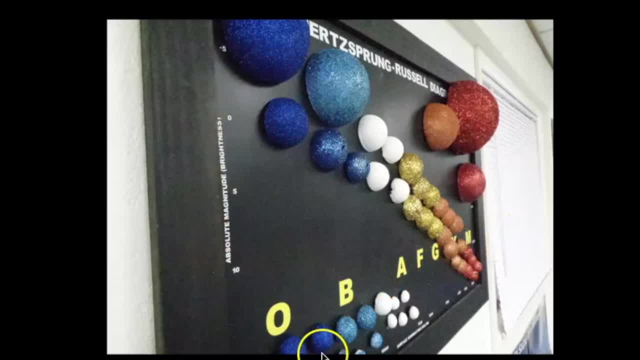 spectral class here, along with magnitude and temperature and color. So when I'm testing my students about this, I like remove all the stars from the magnetic board and I tell them: okay, I want you to put these stars where they should be, And it's just kind of a great way to visualize the HR diagram. I think if I were to do this in the 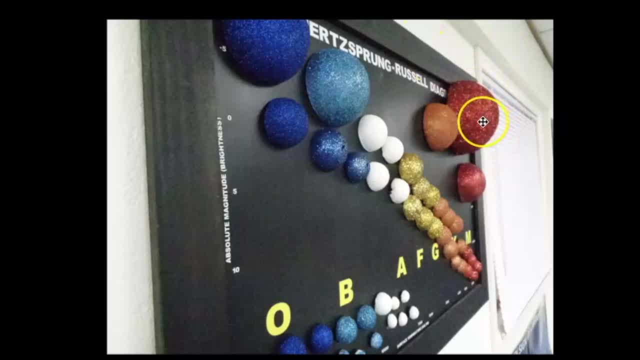 future. I wouldn't cut these in half. I would just have a full sphere and glue some super magnets on it So we can stick the star right on the magnetic board. But it's just another fun project, a great way that I like to make my students build what it is that they are learning. So I hope that this 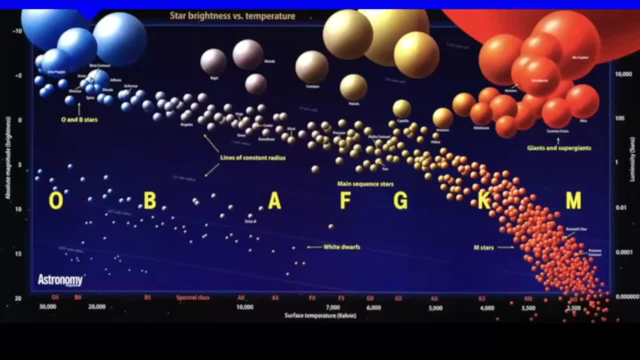 was helpful for you to understand how to read the HR diagram. Remember, here we have main sequence stars. these are stars that are stable. These down here, these are white Dwarf stars, so they're very dim but they're very hot, So that's why they, you know, fall in this temperature range right here. 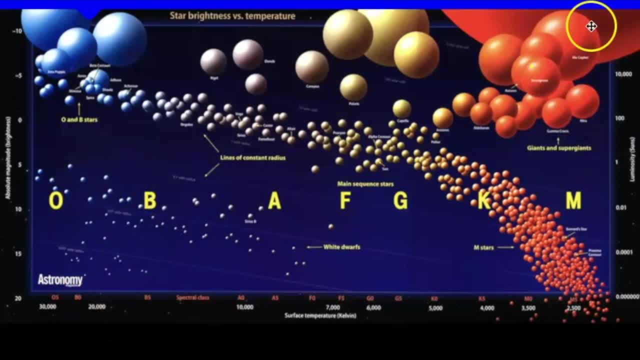 And then stars over here they're very big, or up in this, I should say up in this area- stars are very big, but they can either be ground tanks or they can be right on top of things. So three stars can print out the same color for any node- energy and anygos, and then these can be physically voz and stuff. So this was helpful for the�. 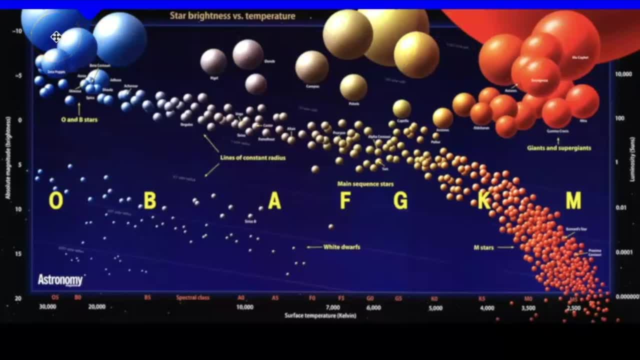 but they can either be cool, they can be medium, well hotter than this, but then they can also be really hot as well. So the position of a star on the HR diagram will change over time, and in a later video I will describe how a star changes over the course of its life and its life really. 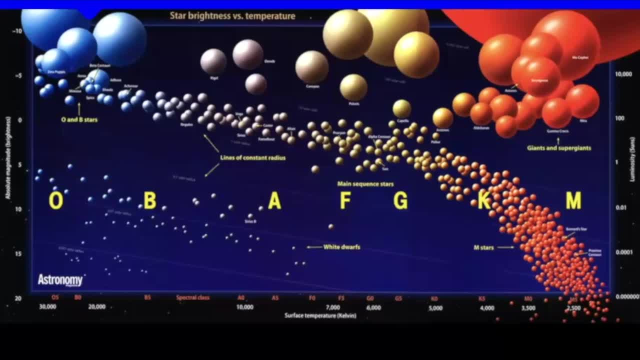 does depend on how big and massive it is. Thank you so much for watching and leave a comment. Do you understand how the HR diagram works and what kinds of questions do you have about it? Thanks again and, as always, keep looking up.